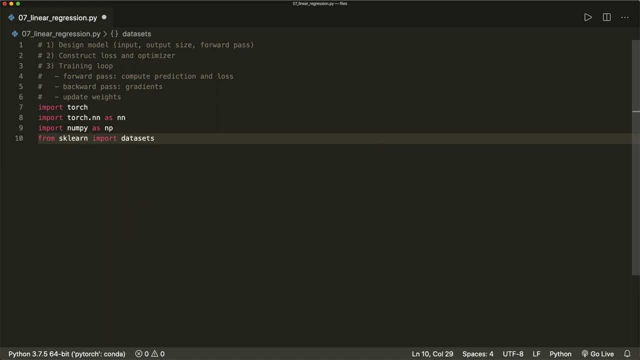 we import data sets to load a binary classification data set, Then from SK learn dot pre process seeing. we want to import standard scalar because we want to scale our features And then from SK learn dot model selection. we import train test split because we want to have a separation. 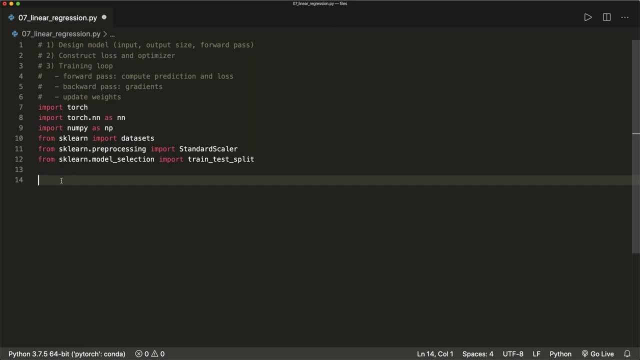 of training and testing data. And now let's do our three steps. So first we want to set up the model, then we want to set up the loss and the optimizer And then, in the third step, we do the actual training loop. 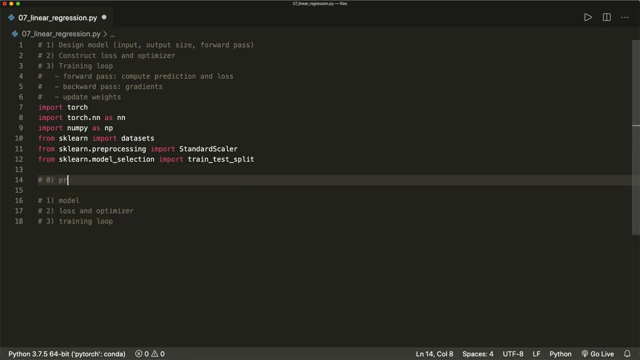 And as a step zero, we want to prepare the data. So let's do this. So let's load the breast cancer data set from SK learn So we can say BC equals data sets. dot load breast cancer. This is a binary classification problem where we can predict cancer based on the input features. 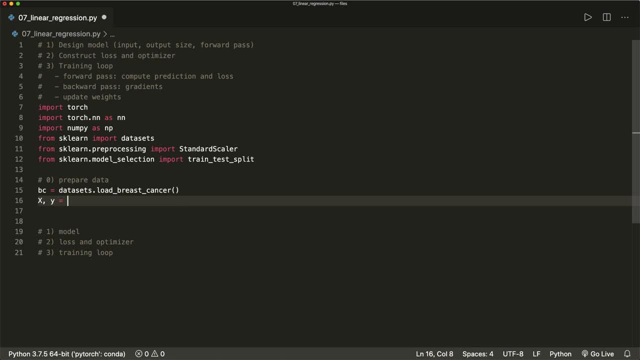 So let's say X and Y equals BC dot data and BC dot target. And then we want to say: well, first of all, let's get to get the number of samples and the number of features by saying: this is X, X, X. 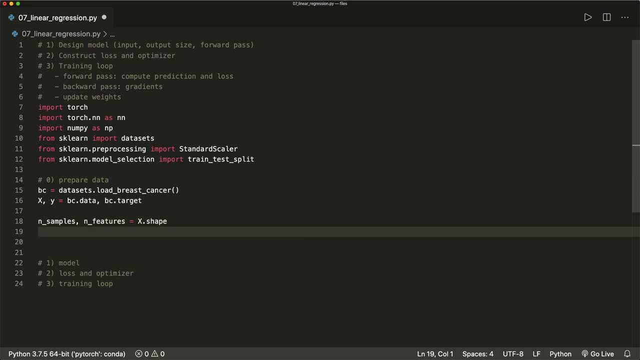 X dot shape. So let's print this first. So print the number of samples and the number of features to see how our data set looks like. And we see we have 569 samples and 30 different features. So a lot of features here And now let's continue And let's split our data when we say x train. 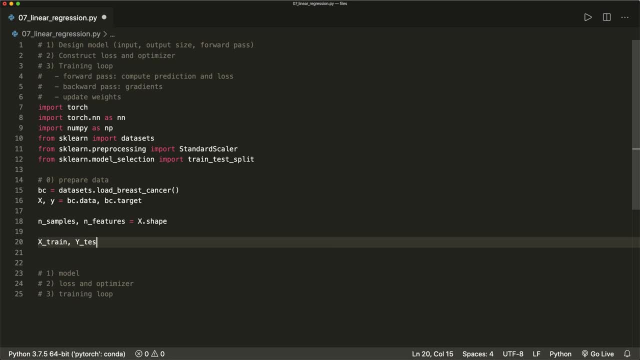 and x test and x test and y, train and y test equals. here we can use the train test split function, where we put in x and y, Okay, Okay, Okay, Okay, And we want to be the test size to be 20%. So this is point two, And let's also 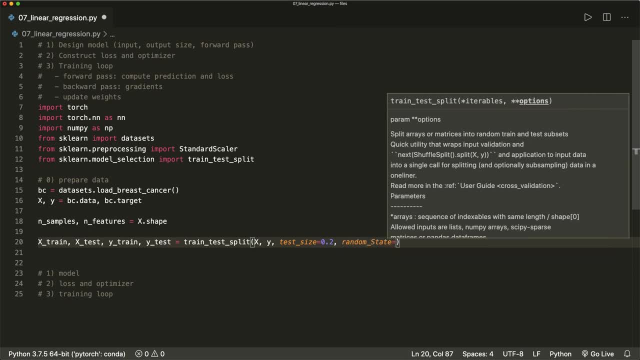 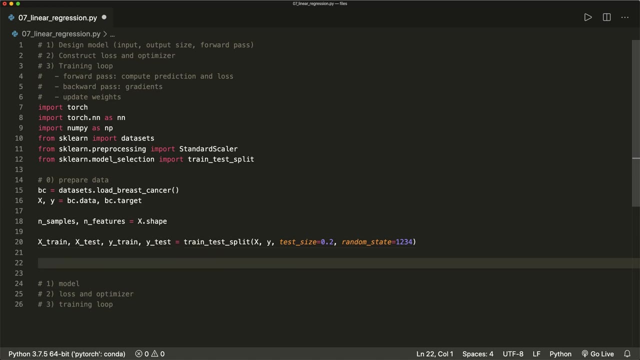 give this a random state equals, let's say, 1234.. And this should be a small s. And now let's convert. or first of all, now we want to scale our features, scale them. here we set up a standard scaler- SC equals standard scaler- which will make 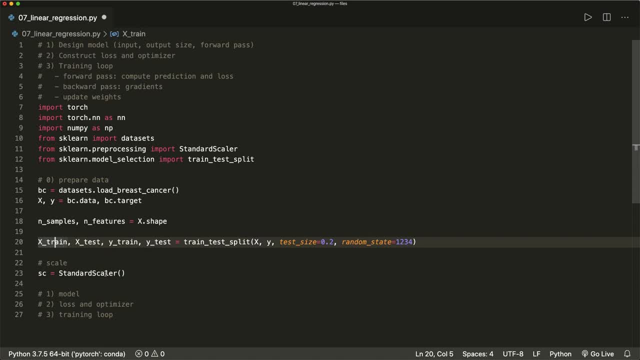 our features to have zero mean and unit variance. This is always recommended to do when we want to deal with logistic regression. So now we scale our data, So we say x train equals s, c, dot, fit, transform, And then as an input we put in x train, And then we want to do: 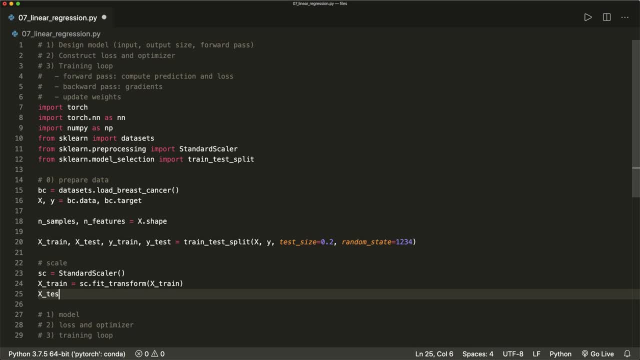 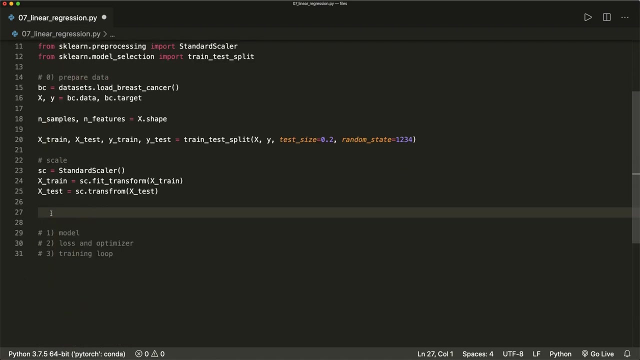 the same thing with our test data. So we say x test equals sc, Here we only transform it And here we put in x test. Now we scaled our data. Now we want to do it with our test, want to convert it to torch tensors. So let's say x train equals torch dot, and here we can. 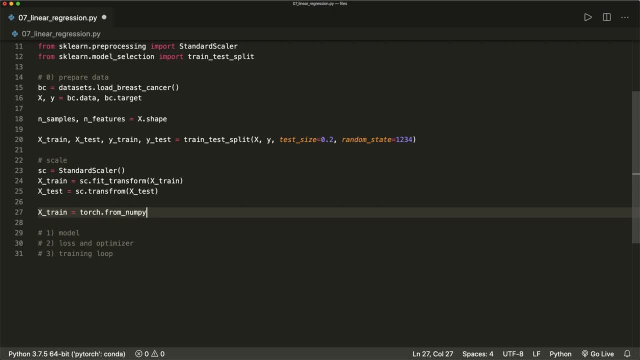 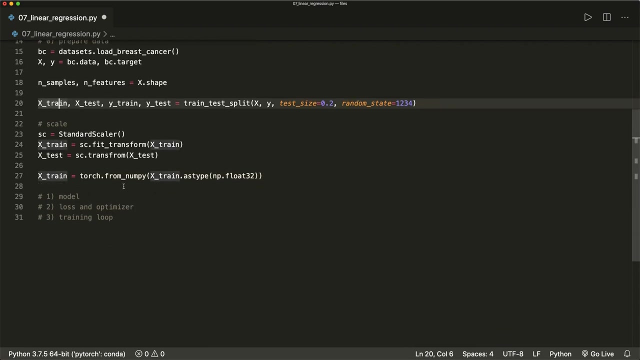 use the function from numpy And then we put in x train and cast this to a float 32 data type. So we say x train dot s type numpy dot, float 32.. Because right now this is of type double and then we would run into some errors later. So let's cast this and convert. 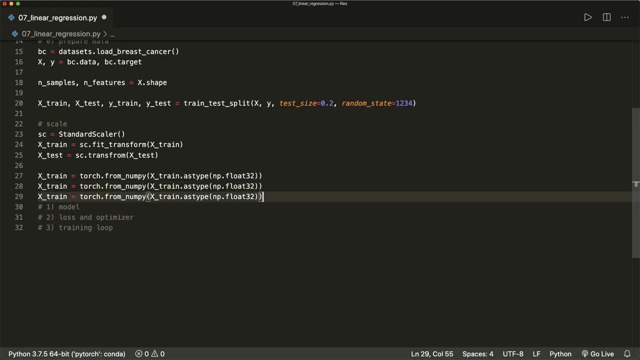 this to a tensor. And now let's do this with all the other arrays. So let's say x test equals this, And our y train and also our y test tensor, Why test? And now, as a last thing to prepare our data, is to reshape our y tensor. So why train equals y train dot view. 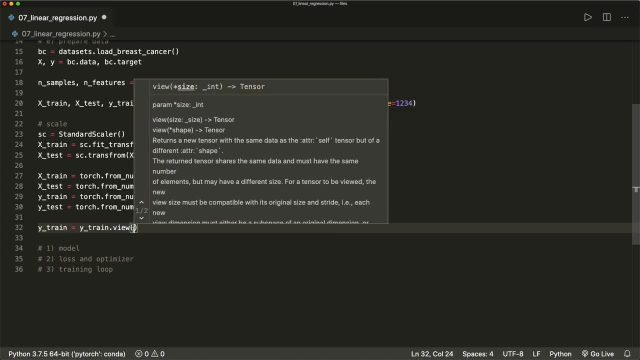 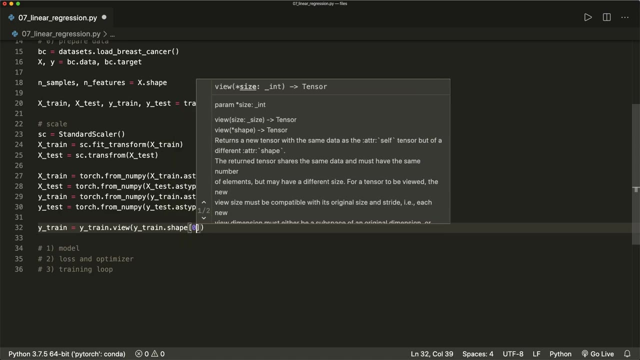 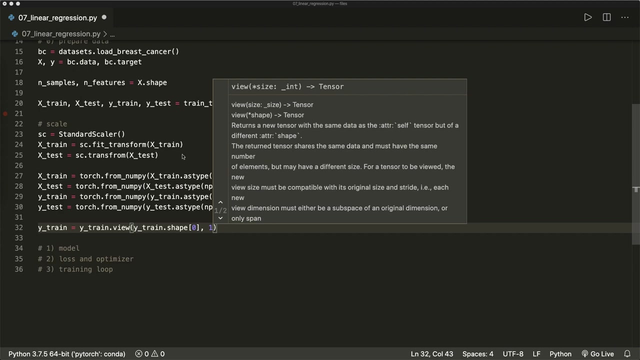 This is a built in function from PyTorch that will reshape our tensor with the given size, So it gets the size y, train dot shape, zero and one. So right now our y has only one row And we want to make it a column vector, So we want to put each value in one row And 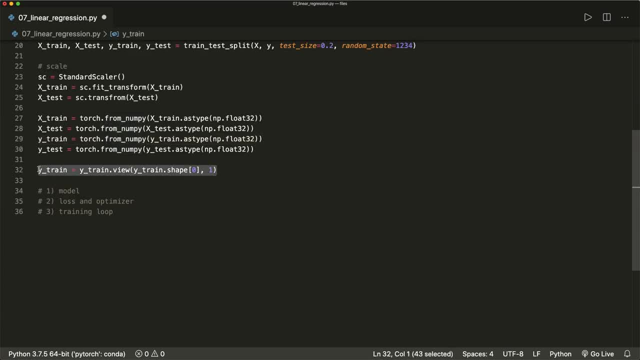 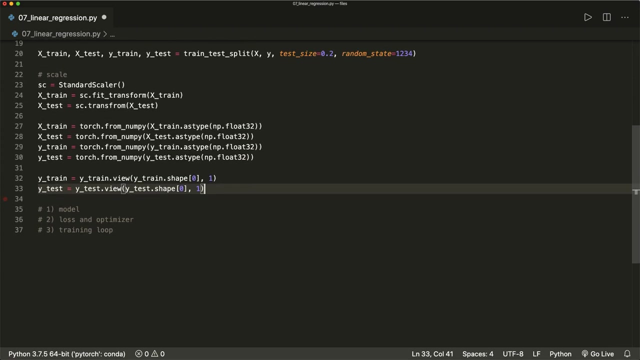 we want to make it a row with only one column, So this will do exactly this, And also for our y test. So y test equals this y test. And now we are- think we are- done with our data preparing. So now let's set up our model, And here our model is a model, And here we. 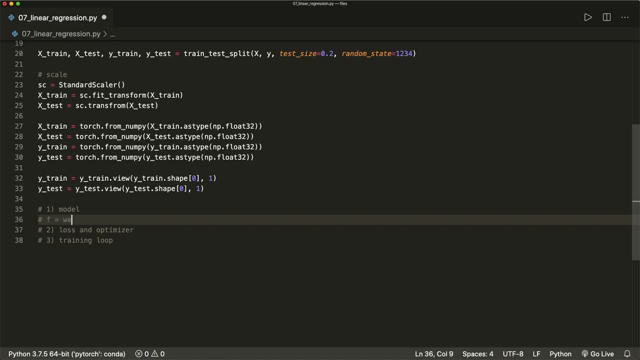 have a logistic regression And we want to write our own class, So let's call this model. Or we can also call this logistic regression Just tick regression, And then we can also call this logistic regression, And then we can also call this logistic regression. And. 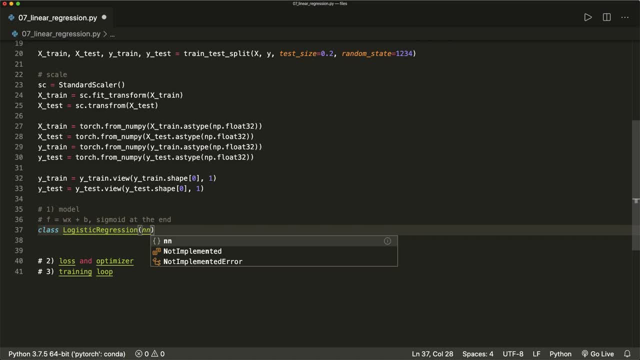 then we can also call this logistic regression, And this must be derived from nn dot module, And then this will get a init which has self, and then it gets the number of input features, And here first we call the super in it. So let's say super. 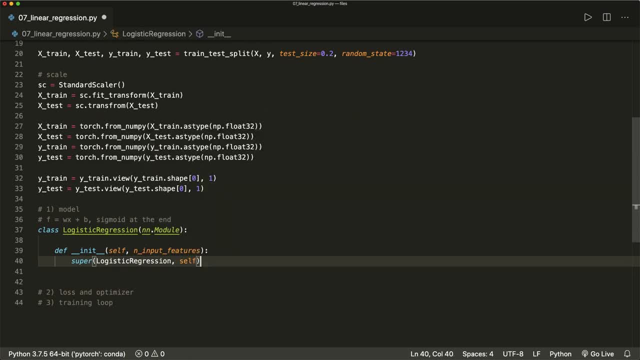 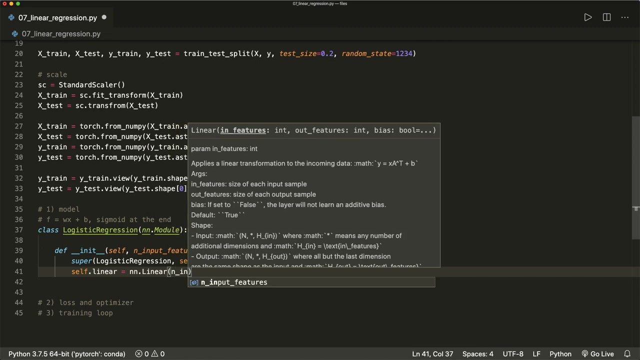 logistic regression and self dot in it. And then here we define our layer. So we only have one layer, self dot linear equals, and here we can use the built in layer and n dot linear, And this gets the input size. So an input features and the output size is just. 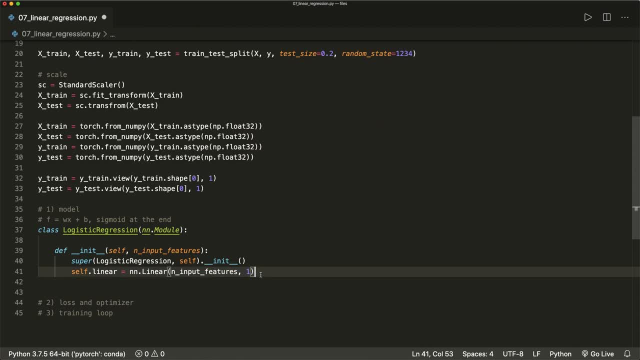 one. So we only want to have one value, one class label at the end. And then we also have to implement the forward pass here, which has self and the data. And our forward pass is: first we apply the linear layer and then the sigmoid function. So here we say, y predicted. 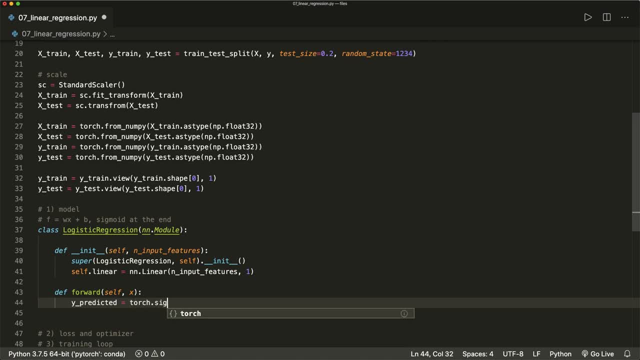 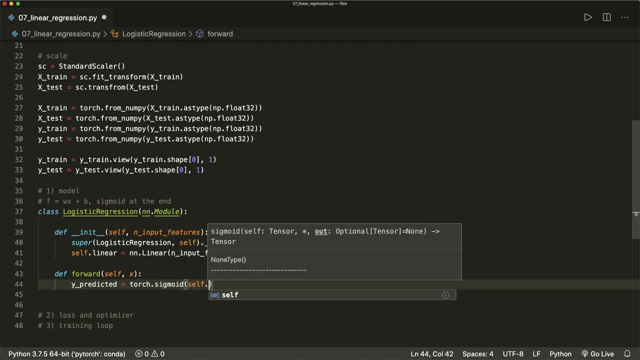 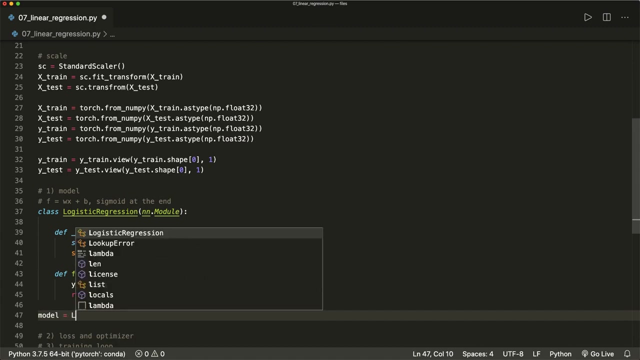 equals torch dot sigmoid. So this is also a built in function that we can use, And here we apply our self dot linear layer, so linear layer with our data x, and then we return our y predicted. So this is our model, And now let's create this model. equals logistic regression of size. 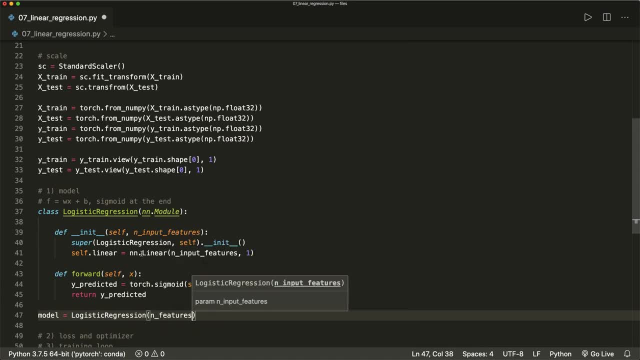 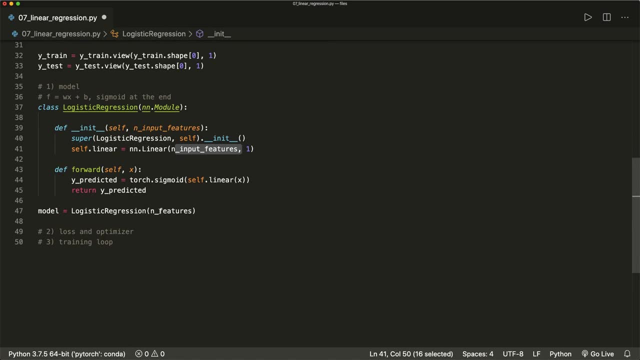 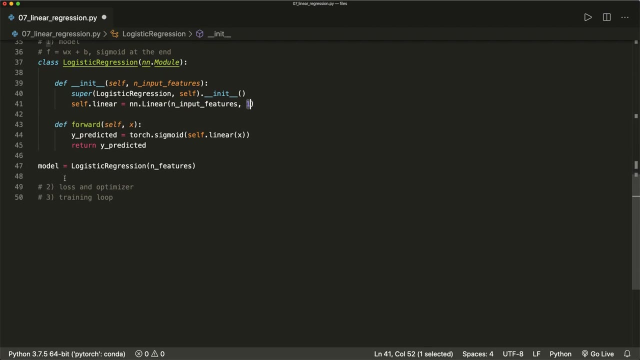 And here we put in the number of features that we have. So now our layer is of size 30 by one, And no sorry, 30 input features and one output feature. And now we have our model And now we can continue with the loss and the optimizer. 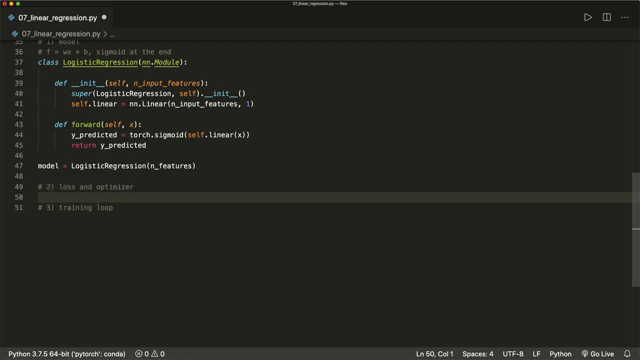 So for a loss the loss function now is different than in the linear regression case. So here we say criteria Y equals and n dot b, c loss. So the binary cross entropy loss here And our optimizer is the same. So this can be. 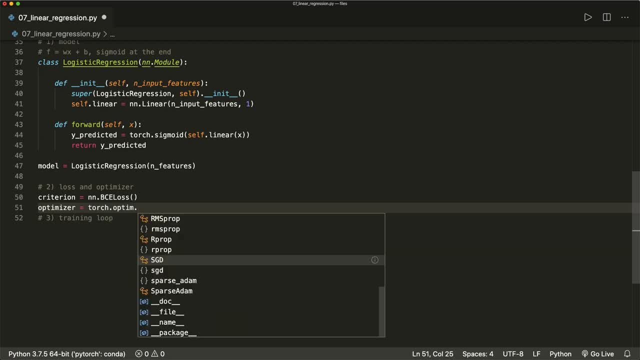 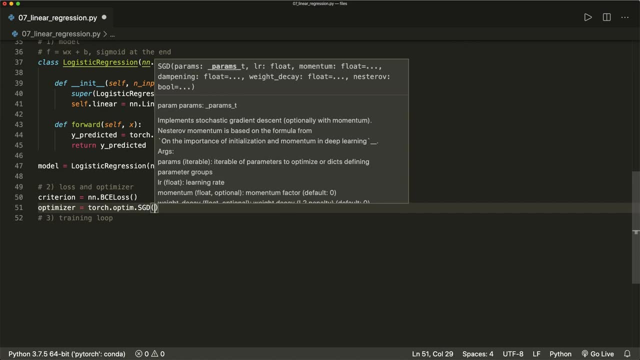 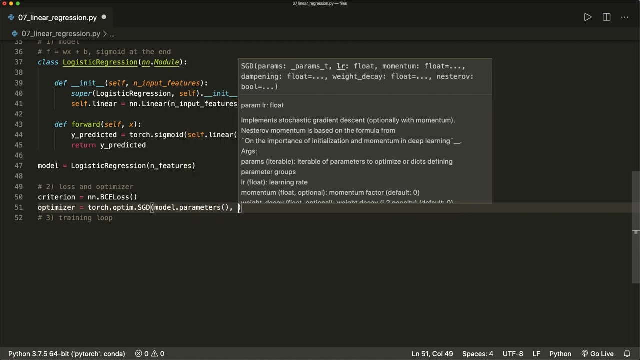 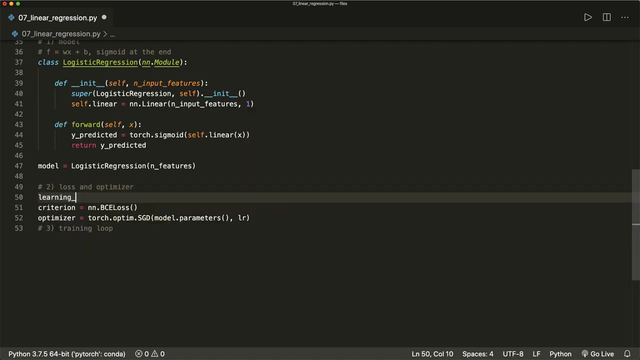 this is torchoptimsg d for stochastic gradient descent, And this gets some parameters that we want to optimize. So here we just say model dot parameters, And it also needs a learning rate. So let's say our learning rate equals point 01.. And then here we say l r equals learning rate. 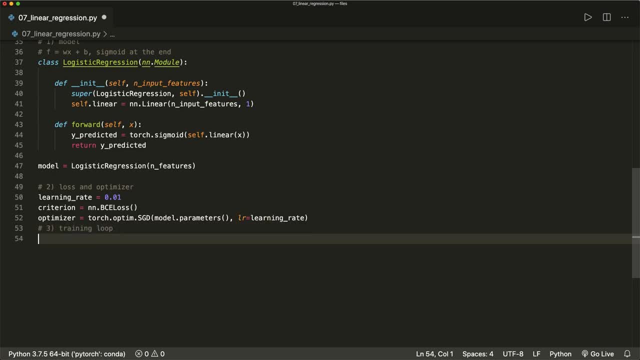 So now this is step two and now step three. So let's define some number of epochs equals, let's say, 100 iterations, And now we do our training loop. So now we do for epoch in range num epochs, And then first we do the forward pass, forward pass and the loss calculation. 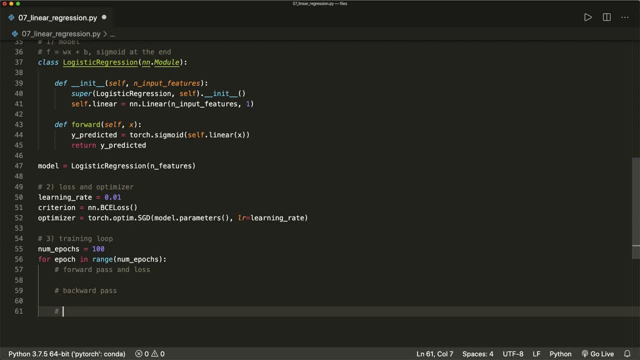 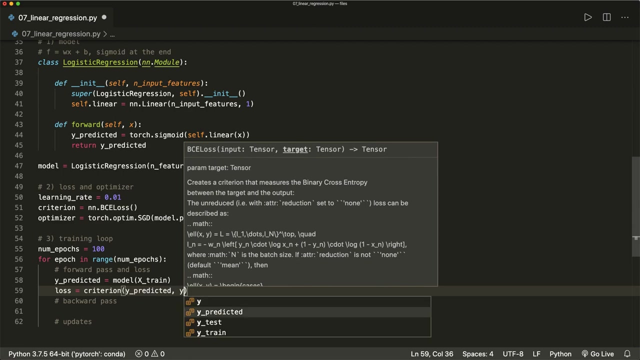 Then we do the backward pass And then we do the updates. So let's say: y predicted equals. here we call our model And as data it gets x train. And then we say loss equals criterion And this will get a, the y predicted and the actual y training. 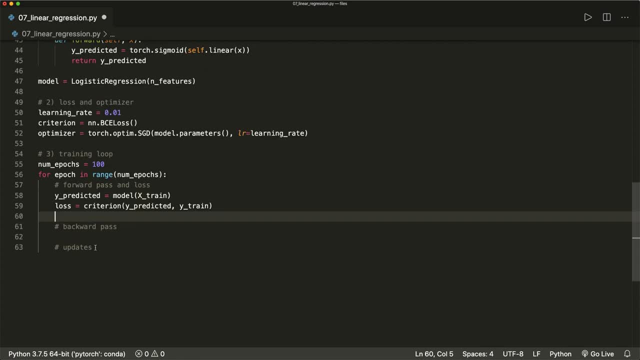 So the training samples or training labels, And now we do the backward pass and calculate the gradients, And again we simply have to call lost, dot, dot backward, and pytorch will do all the calculations for us. And now we update our weights. So 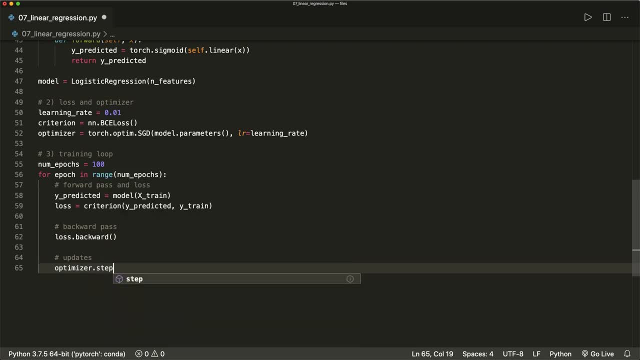 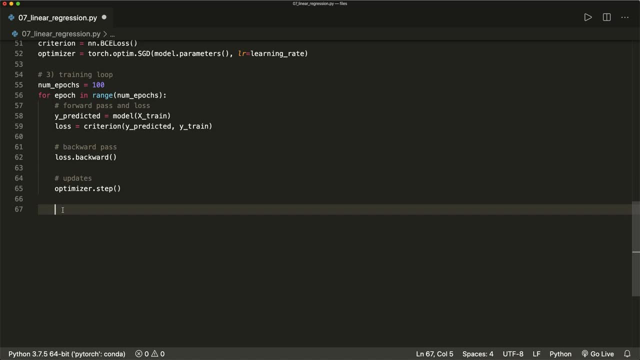 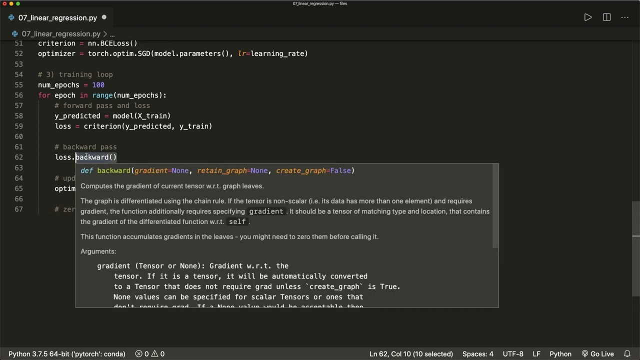 here we simply have to say optimizer, dot, step, And again pytorch will do all the update calculations for us. And then we don't want, we must not forget to empty our gradients again. So onto zero the gradients, because the backward function here will always add. 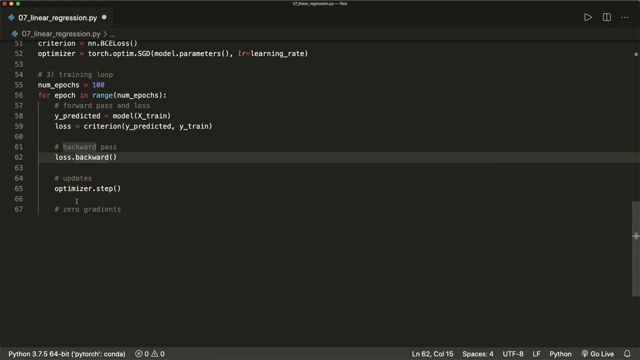 up all the gradients into the dot grad attribute. So let's empty them again before the next iteration And we simply must say optimizer dot, zero grad. And then let's also print some information. if E, POC plus one, modulo 10 equals, equals zero. So every 10th step we want to print some information. let's 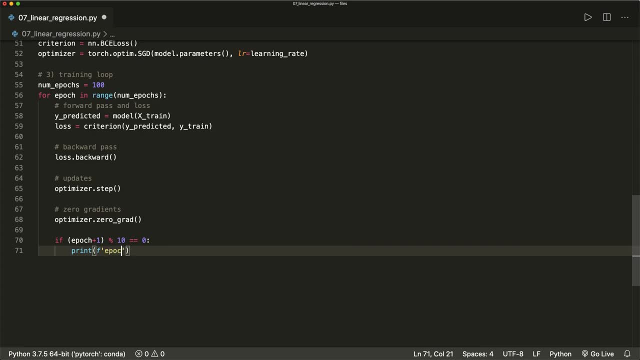 use an F string. here Let's say epoch, And here we can use epoch plus one. And then we also want to see the loss. So the loss equals loss dot item. And let's format this to say: to only print four decimal values. And yeah, so now we are done. This is our logistic regression. 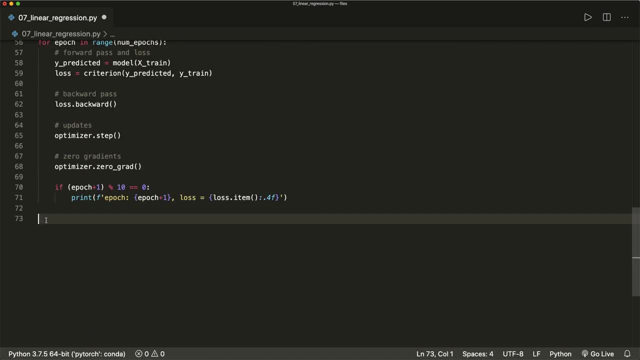 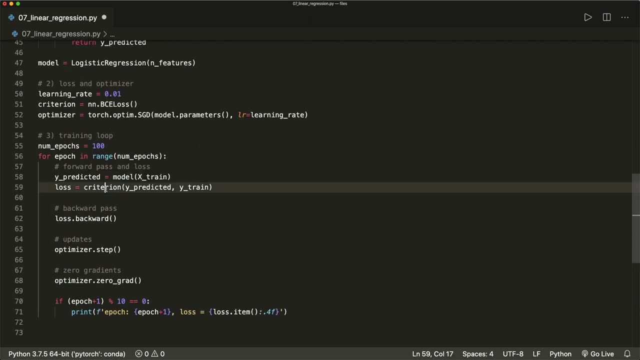 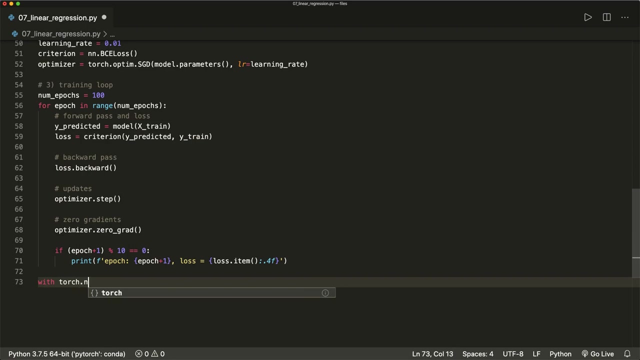 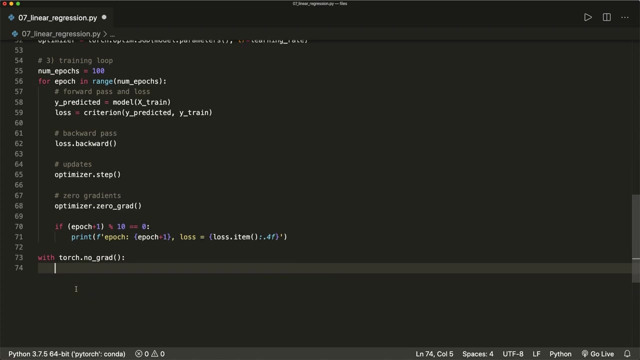 implementation. And now let's evaluate our model. So the evaluation should not be part of our computational graph, where we want to track the history. So we want to say with torch dot, no grad, and then do our evaluation here. So here I want to get the accuracy. 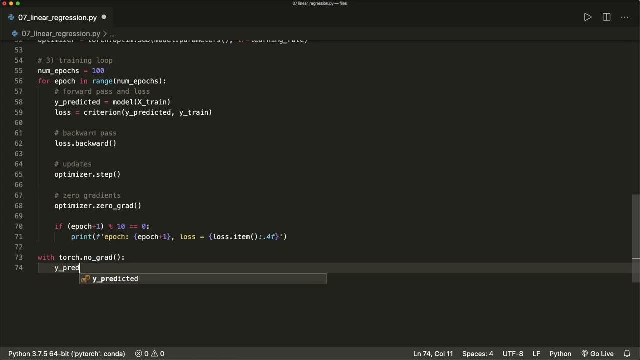 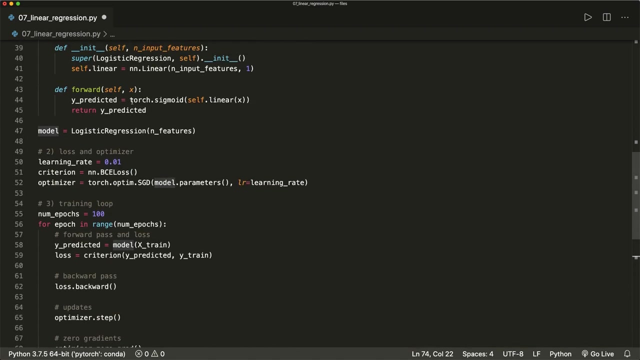 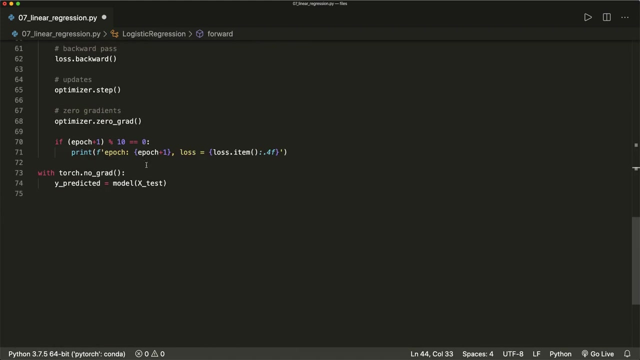 So let's get all the predicted classes from our test samples. So let's say this is model And here we put in an x test, And then let's convert this to class labels. So zero or one. So remember, the sigmoid function here will return a value between zero and one, And if this is larger, 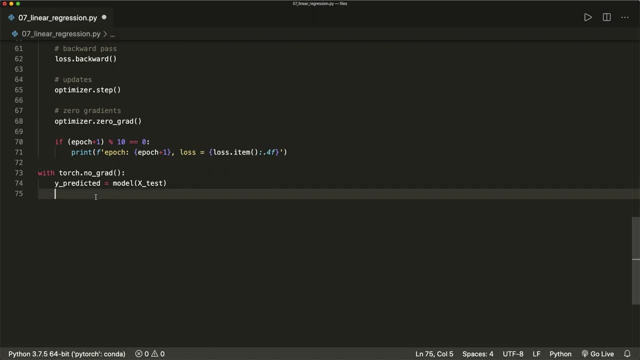 than point five. we say: this is class one and otherwise it's class zero. So let's say: y predicted classes equals. why predicted dot round? So here we can use a built in function again And this will do exactly this. And yeah, so if we do don't use this statement, then this would: 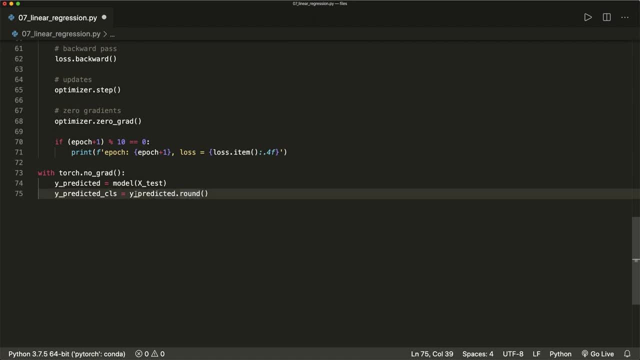 be part of the computational graph And it would track the gradient calculations for us. So here, we don't want this. we don't need this because we are done. So that's why we use this with statement here And now. let's calculate the accuracy by saying: AC equals. 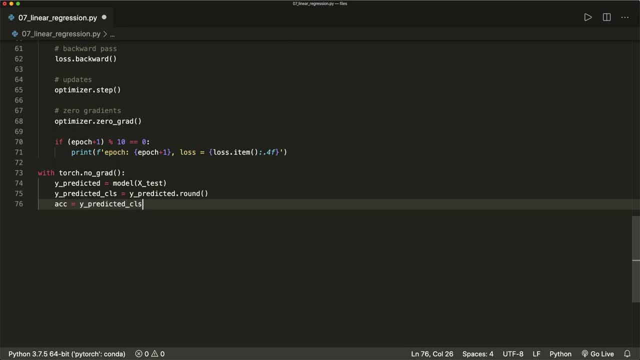 y predicted classes, And here we can call the equal function equals y test, And then the sum. So we want to sum them up: for every prediction that is correct, it will add plus one, And then we divide this by the number of samples, of test samples. So why test dot? 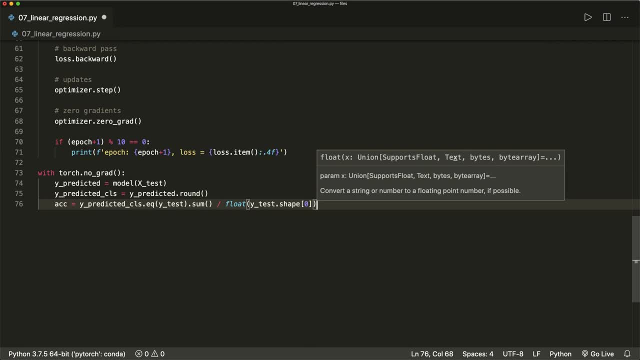 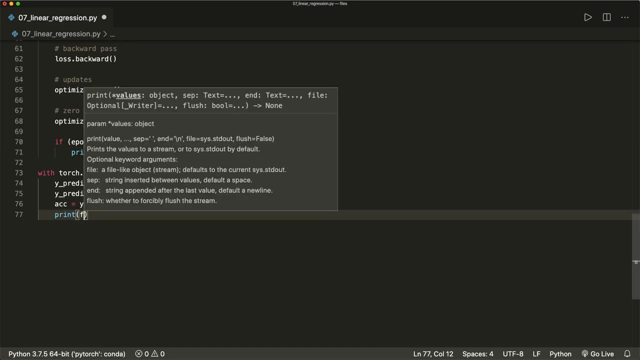 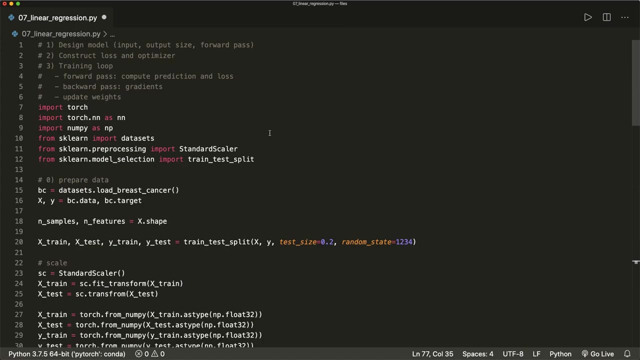 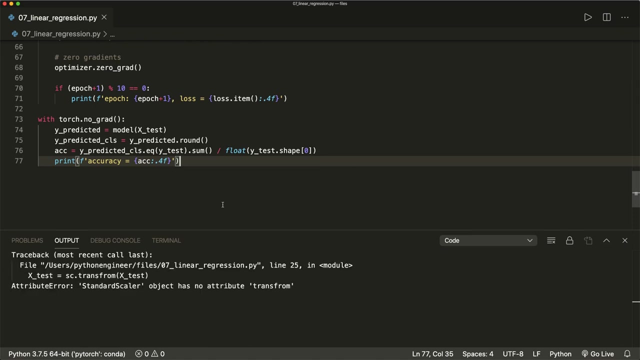 shape zero. this will return the number of test samples. And then let's print our accuracy. print accuracy equals x dot point four, f, also only four decimal values. And now let's run this and hope that everything is correct. And standard scalar has no attribute trans from. So here I have. 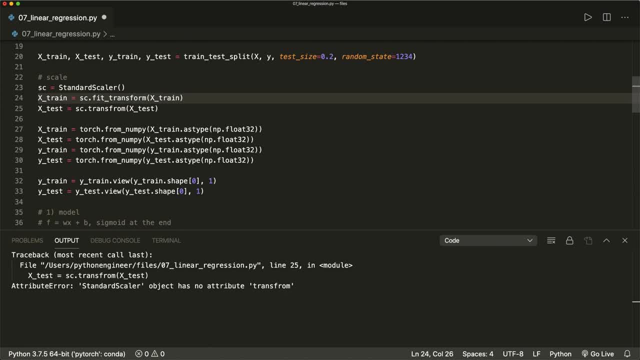 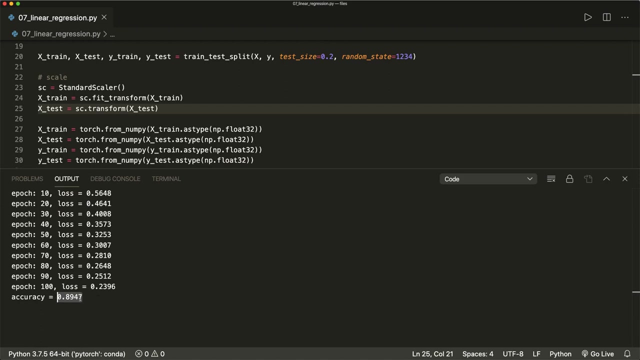 a typo. Transform Now let's run this again. Trans form One more try And now we are done And we have a accuracy of point 89.. So it's okay, it's good, but it's not perfect. So you might want to play around with, for example, 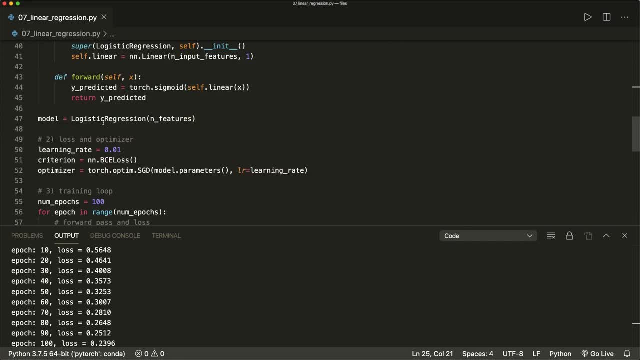 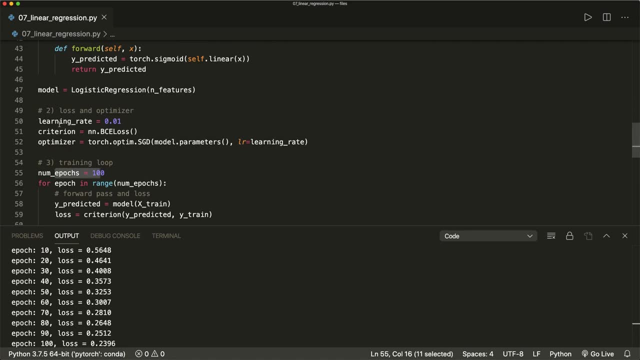 the number of iterations And where do we have it- The number of epochs or the learning rate, for example, or also maybe try out a different optimizer here. But basically that's how we implement logistic regression. I hope you liked it. If you liked it, please subscribe to the channel and see you next time. Bye.